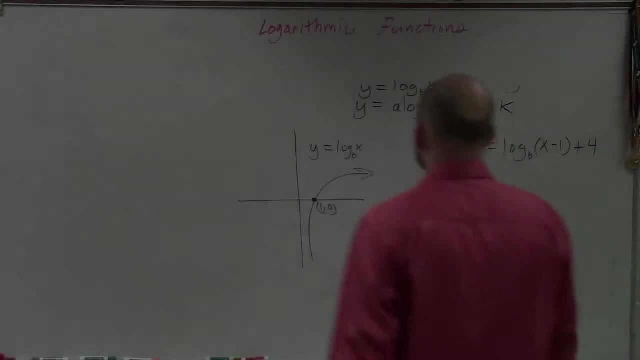 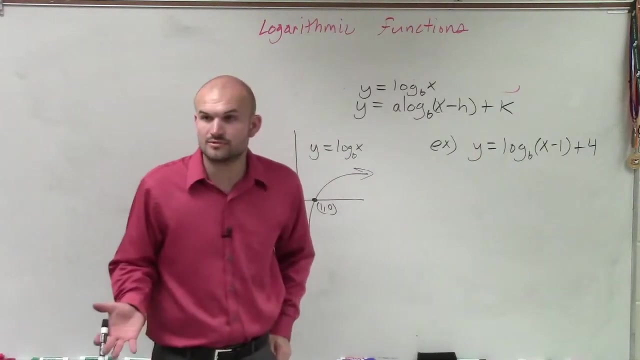 All right. First of all, the main important thing is you take your exponential right and then we just go ahead and determine what would be some two points that we could use for this. So, again, we could create a table if we wanted to, but creating a table is. 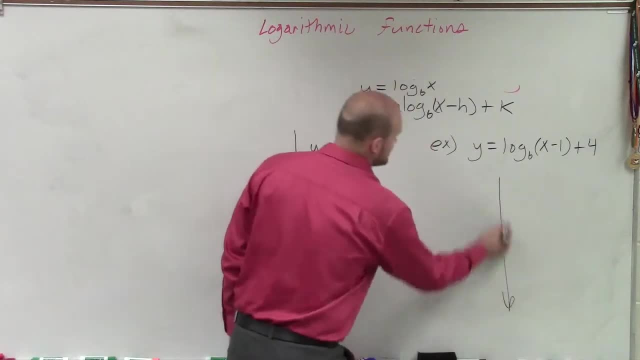 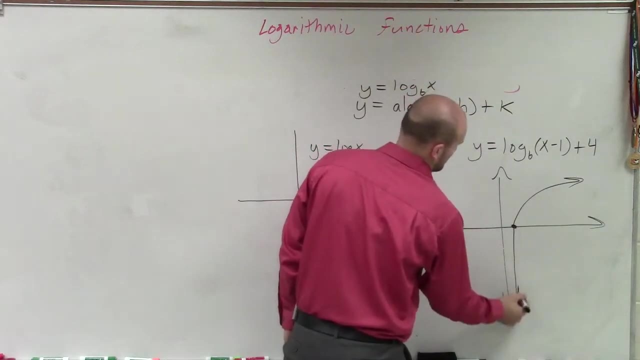 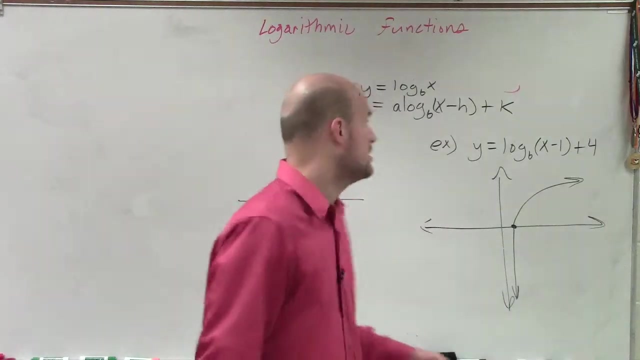 to me it's just going to be a lot of extra time. So all I'd like you guys to do is just plot the parent graph And then, once plotting the parent graph, now what we're simply going to do is go and take a look at the transformations. Well, you can say the transformations, for 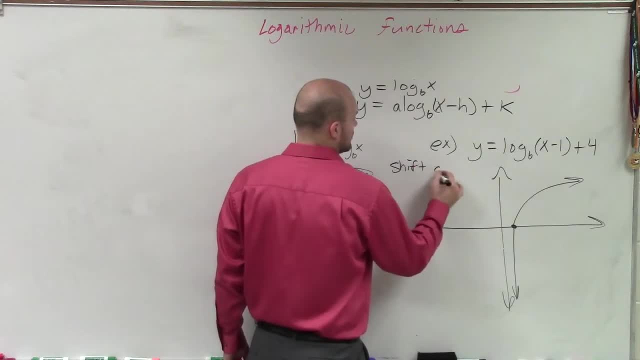 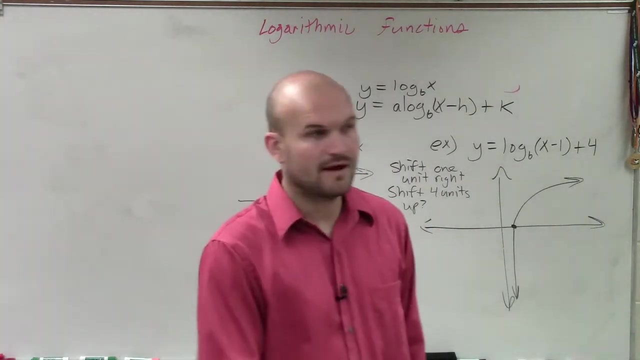 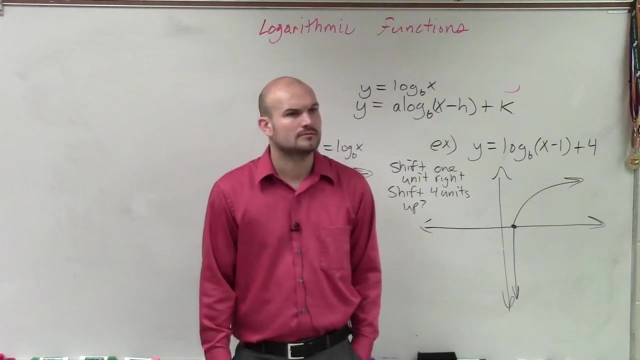 this graph is: you're going to shift one unit to the right and shift four units up, And then you're going to野ronize it lot. All right, Thank you, Yeah, Yes, I thought there was a. Is it earlier release today? 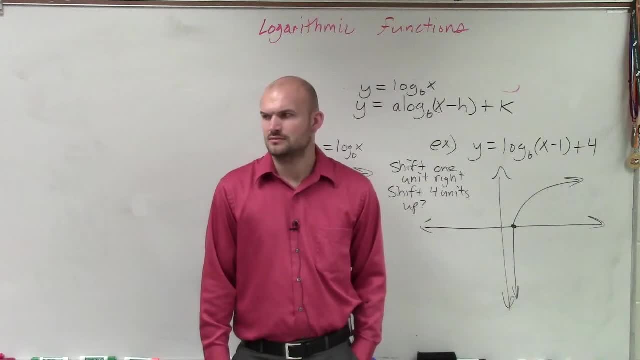 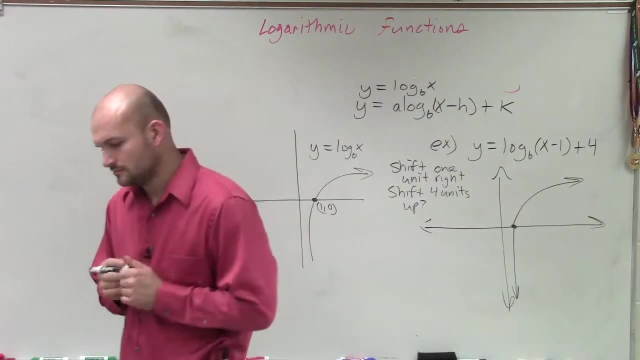 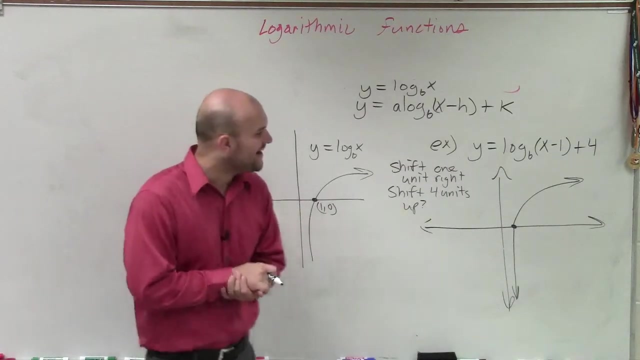 Yeah, last week. Teachers, please disregard the last bell Again. please disregard the last bell. All right, Can you do it? I don't see it. Yeah, Oh, we're still going. OK, So now, what we're simply going to do is: now you guys can. 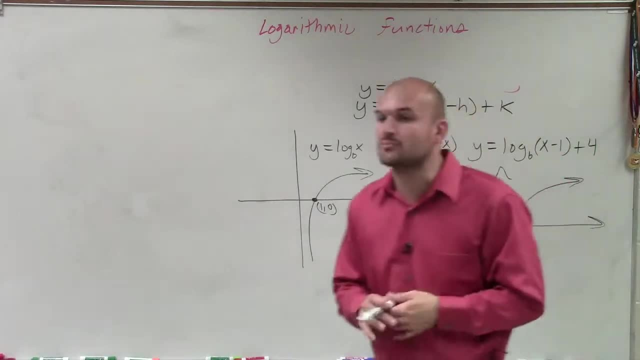 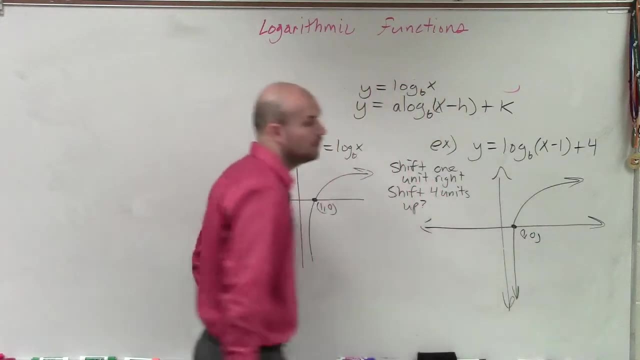 and this is all I'm really going to expect. You could be able to find another point to look through, but now you guys just need to take this, And the one point we know that we have that we figured out was 1 comma 0, right. 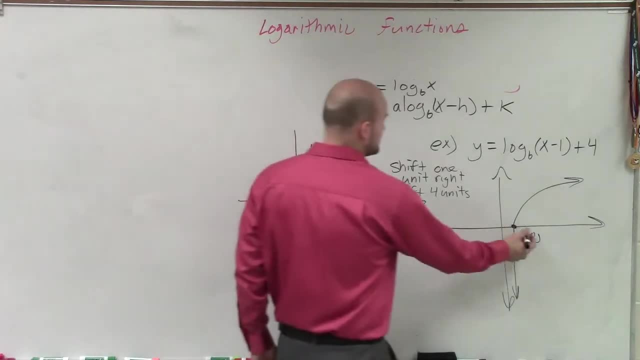 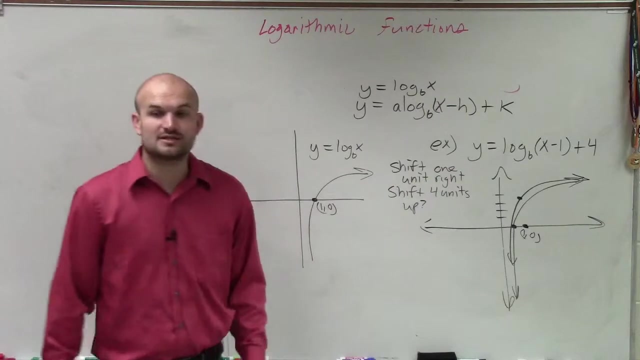 So now we just need to shift that one unit to the right and then four units up: 1,, 2,, 3, 4.. All right Now there is a couple of differences, though, that you guys are going to need to determine. 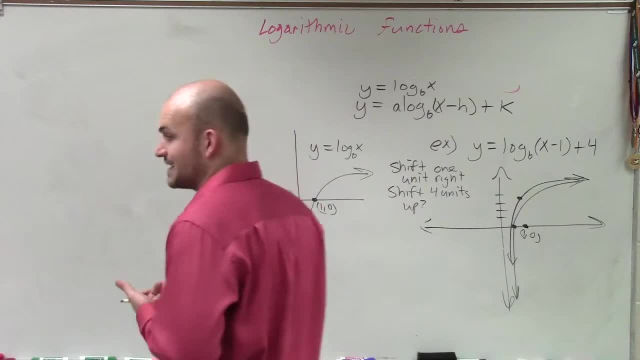 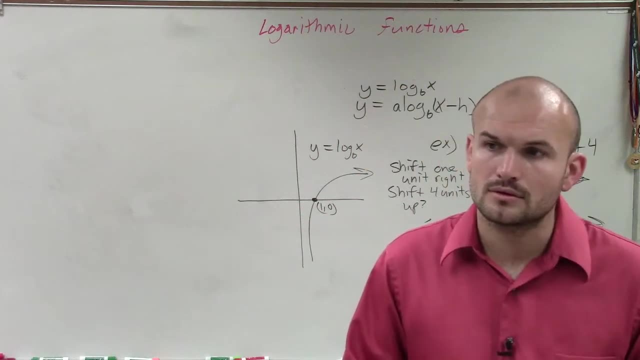 We do need to make sure that we are able to determine the x-intercept. Yes, If it's just one of the same spots, is it true that we have the same spot on the x-intercept? It's not the exact same spot.